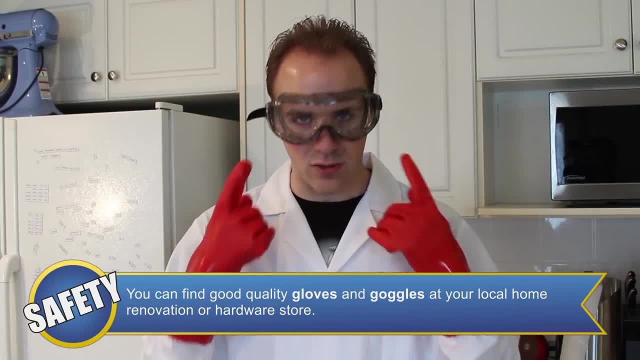 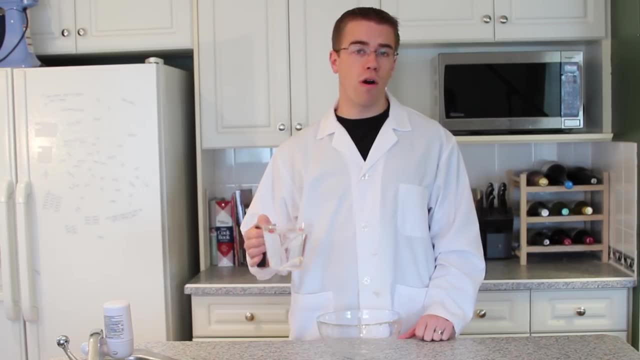 Because we're dealing with boiling water today. the safety equipment we're going to need include goggles, heat-resistant gloves and an apron or lab coat to protect from spills or splashes. The first step in our experiment is to take some cold water and fill up our bowl. 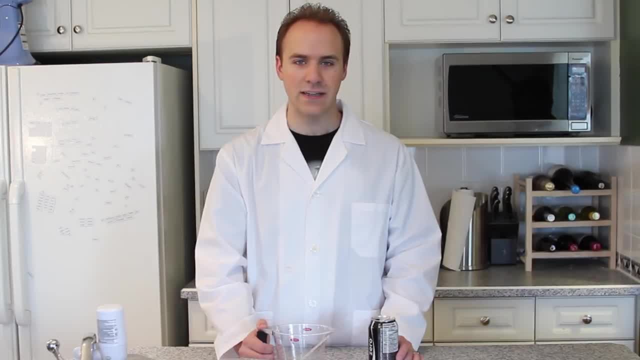 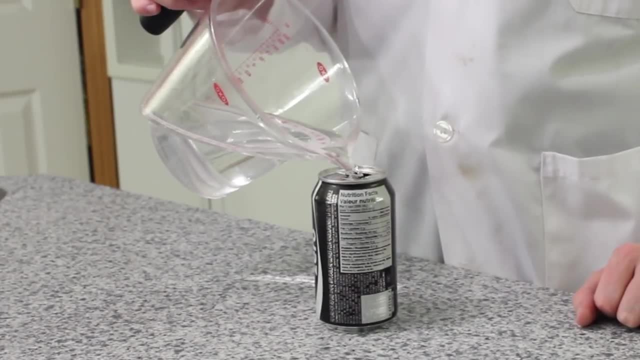 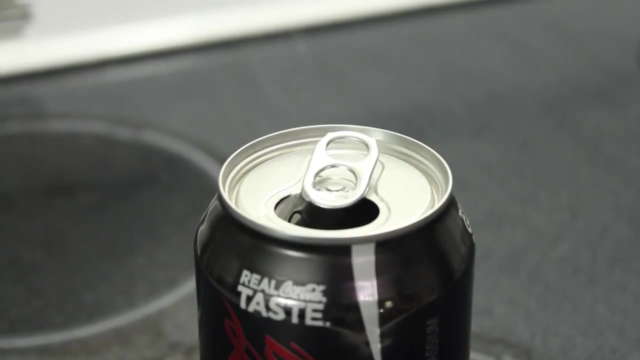 The second step of our experiment is to pour about 100 ml water into the can. Turn your stove to medium-high heat and place your can with the water in it in the center of the burner. Leave it there until you see water vapor coming out at the top. 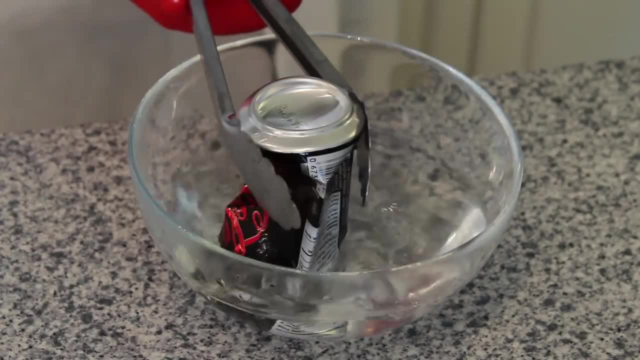 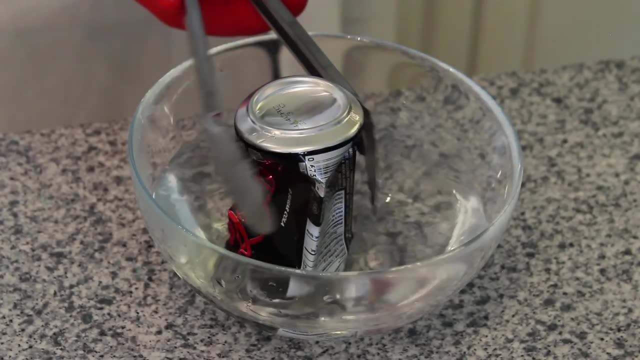 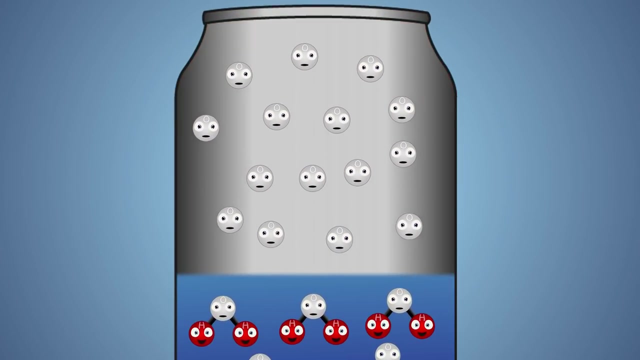 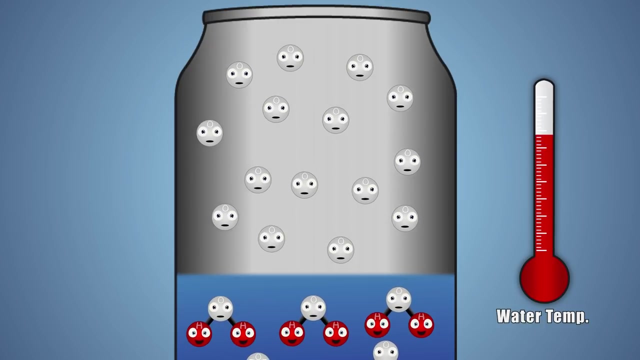 Now quickly dunk your can into the water. Let's look at this experiment a little closer. Before we heat our can, it's filled with liquid water and gaseous air molecules. Heating our can adds energy to our liquid water. The more energy we give our water molecules, the more excited they get and the further 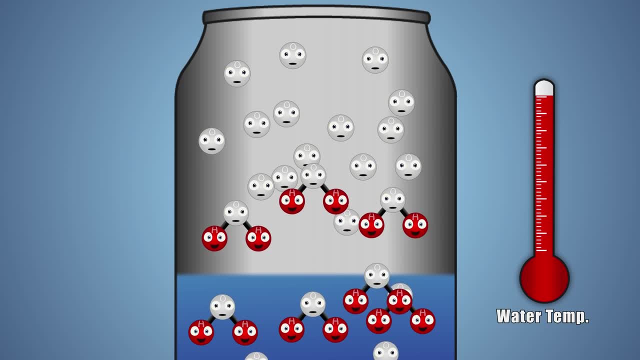 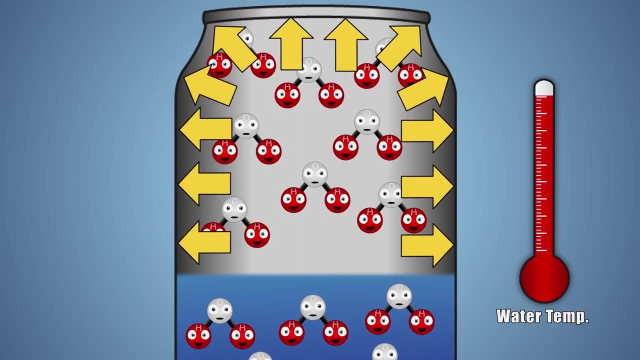 apart the molecules spread. Once enough energy has been added to our liquid water, it changes state from a liquid to a gas. This gas is called water vapor. As our water vapor fills our can, it presses against the sides of our can, creating an 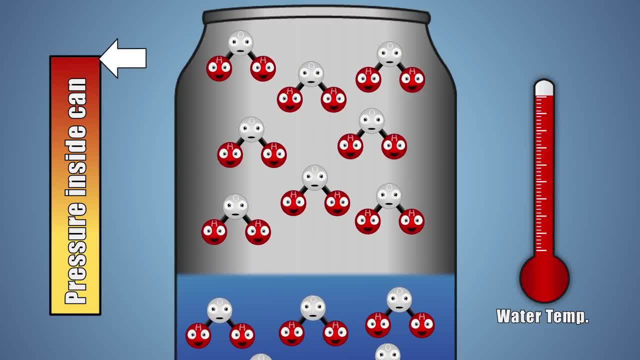 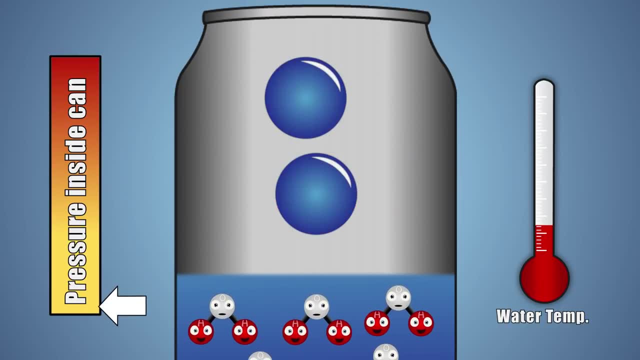 increase in pressure. When we place our hot can upside down in our cold water, all the water vapor molecules that fill our can get really close together and turn into a few drops of liquid water. This liquid takes up a lot less space than a gas. 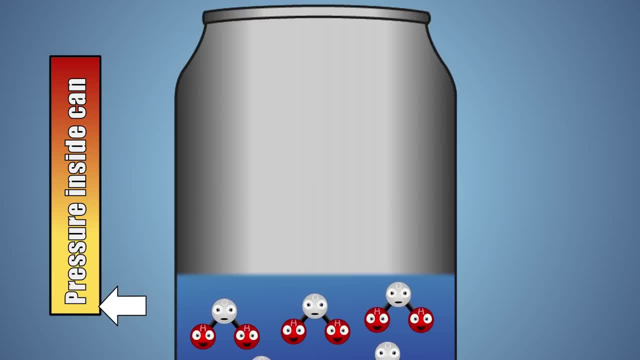 Water in its liquid state doesn't exert nearly as much pressure on the inside of the can as it did in its gaseous state. At this point in our experiment, the outside atmospheric pressure is much higher than the pressure inside the can. In nature, pressures want to be balanced or in equilibrium. 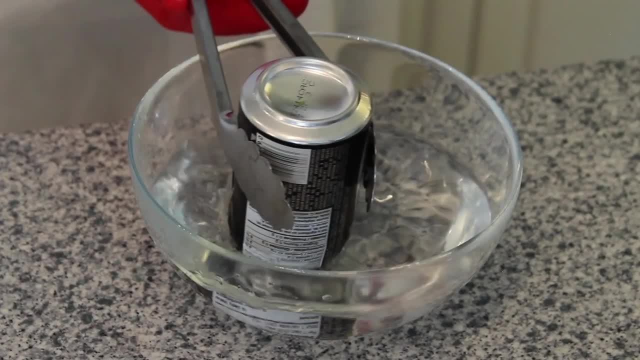 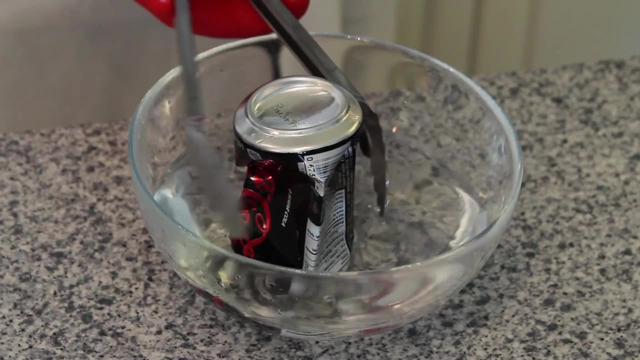 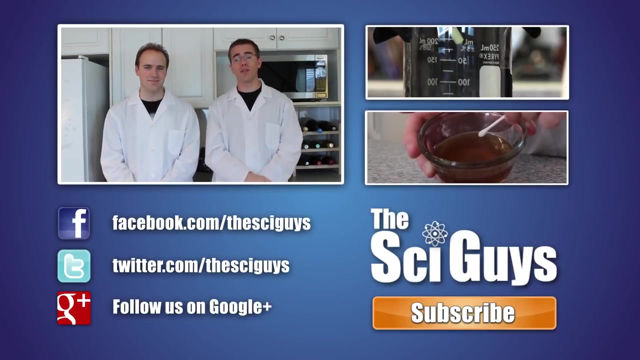 This imbalance causes the can to violent. This violent collapse towards the center of the can is called an implosion. That's it for Can Crushers. I hope you enjoyed it. If you did, drop us a like and a comment below and subscribe for future episodes. 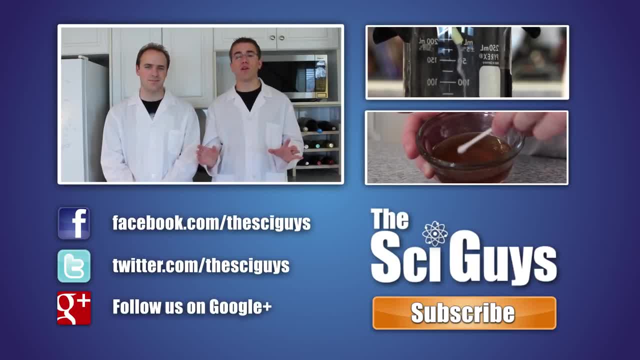 Like us on Facebook and follow us on Twitter, And if you have any questions related to this episode or about science in general, let us know in the comments below or message us on Facebook, and we'll try to help you out as best as possible. 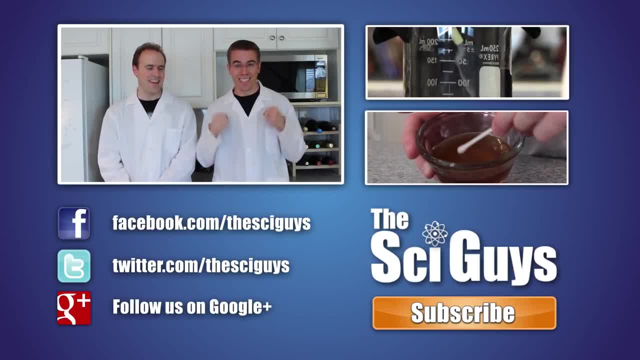 Thanks for watching. Bye, Ryan, got to crush cans. Yeah, you did. Here at Sci Guys, we're always curious how experiments turn out, So if you do these experiments at home, share a video or photo of them with us on our Facebook.